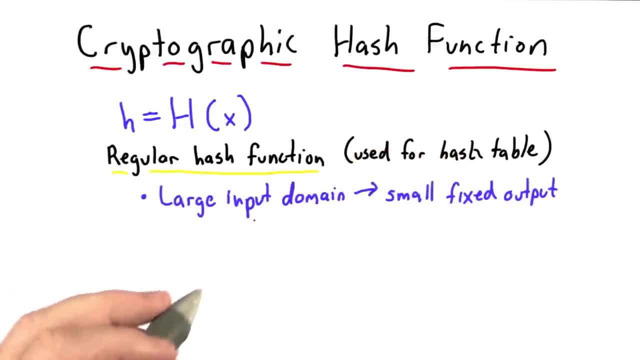 It has the property that it maps values from a large input domain- and by large here we usually mean infinite, such as all possible strings of any length, to a small fixed output size. It should also have the property that it's well distributed. 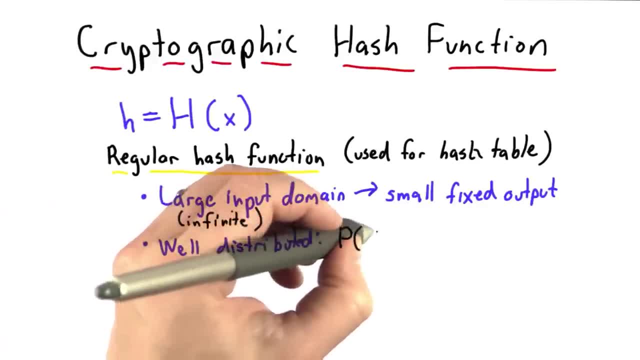 that for any given input, the probability that that input maps to a particular value is close to 1 over the size of the table, And we'll use n to represent the output size. So we'll say that outputs are in the range from 0 up to n. 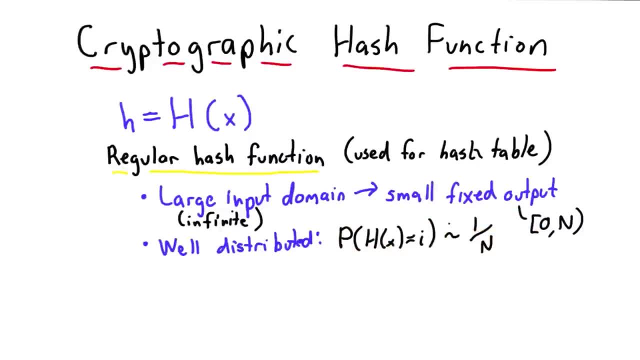 And so if it has this well distributed property, well, this works great for a hash table. This is not enough for cryptographic commitments. If we just had these 2 properties, well, it might be easy to find other x values that map to the same thing. 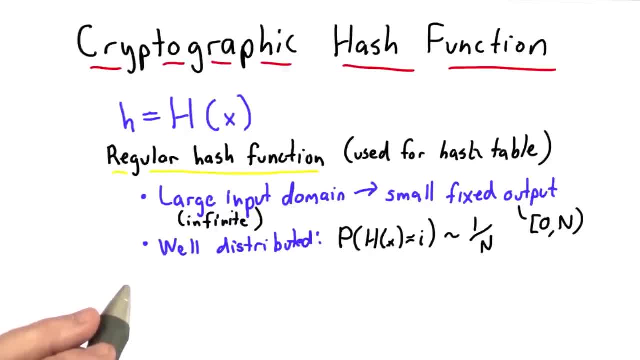 And we saw that one of the things that we need for a cryptographic hash function is to make it hard for Alice to be able to do that. otherwise she could find 2 inputs and cheat in the coin tossing game. This first property of mapping a large input domain to a small fixed output. 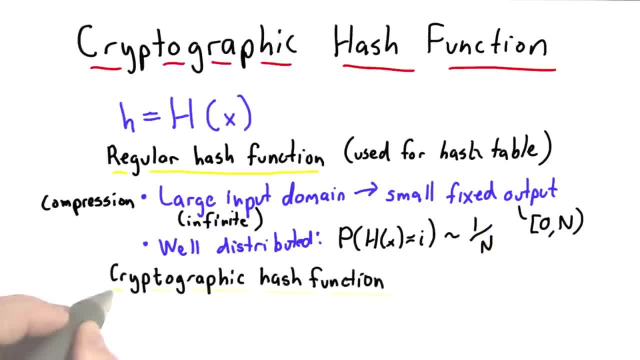 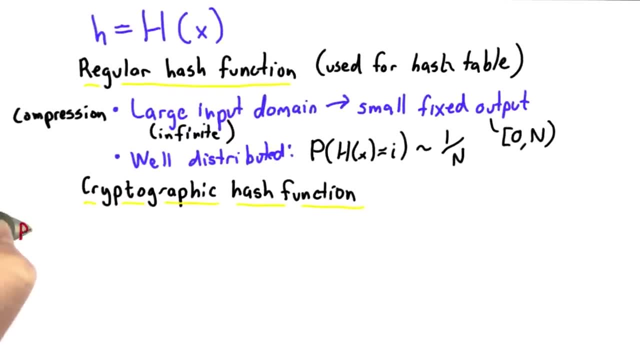 we'll call compression. What we need for a cryptographic hash function is 3 additional properties. The properties are preimage resistance, which means, given the output of the hash function, it's hard to find the input that produced it. This is a form of one-wayness. 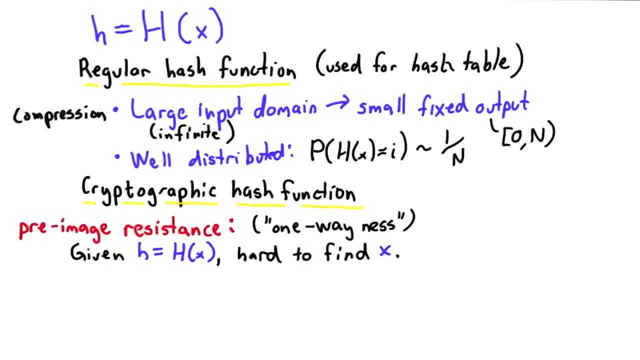 The other 2 properties we need concern the collision resistance. The weakest form of this is known as weak collision resistance. What weak collision resistance means is that if we're given some hash value, it's hard to find any input that hashes to the same result. 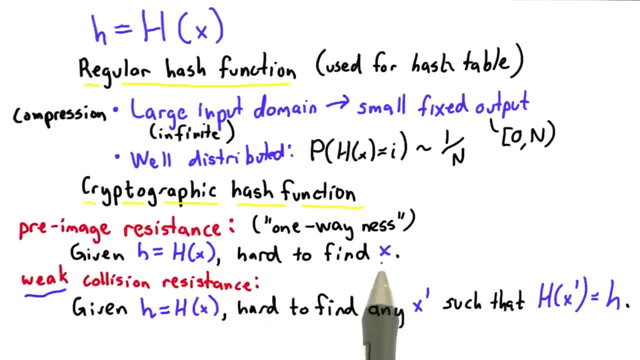 These are sort of similar. This one says it's hard to find the actual value of x that was used. This one says it's hard to find any x prime value that hashes to that value. If we have weak collision resistance, that would imply we have a form of preimage resistance as well. 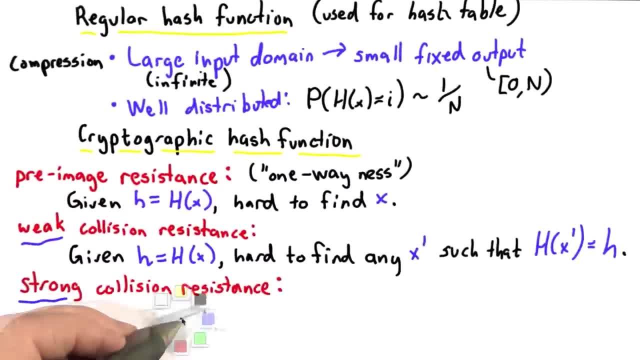 The final property is strong collision resistance, which is exactly the one we saw that we needed for the coin tossing game. Strong collision resistance requires that it's hard to find any pair, x and y, such that the hash of x is equal to the hash of y.